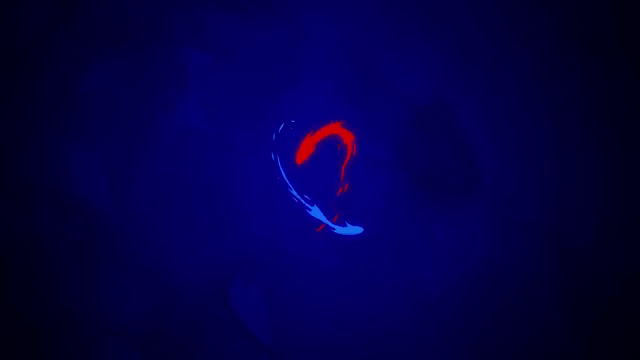 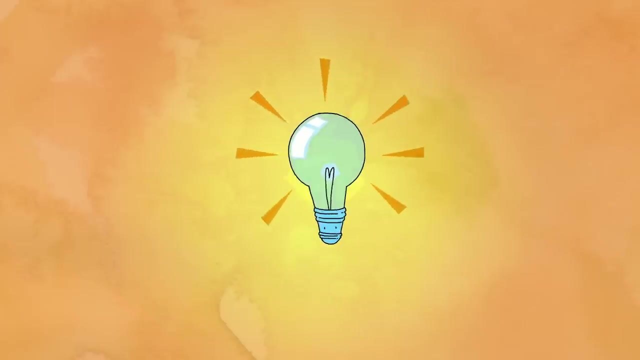 Why it gets dark sometimes. The idea is that very few objects actually emit their own light. The special light-emitting objects like the sun or a lightbulb are known as sources of light. Most of the things we see, like that pencil on your desk, are simply reflecting light from a 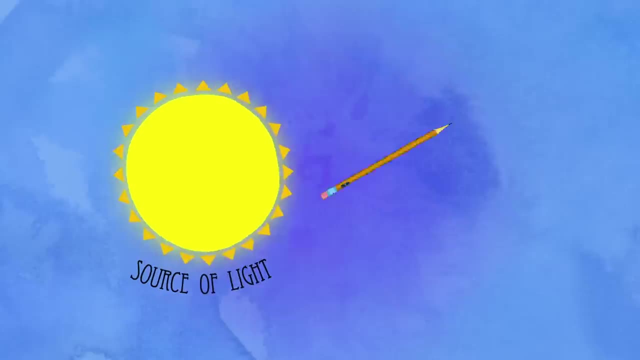 source rather than producing their own. So when you look at your pencil, the light that hits your eye actually originated at the sun and has travelled millions of miles across empty space before bouncing off the pencil and into your eye, Which is pretty cool when you think about it. 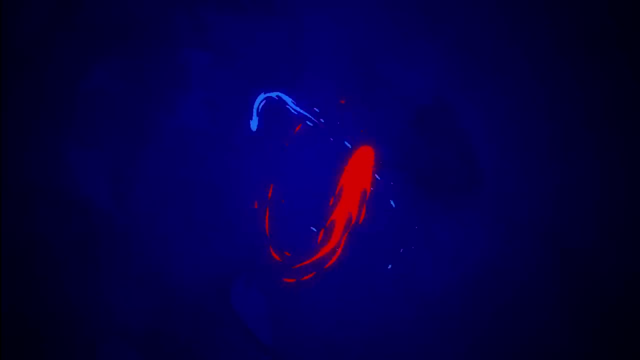 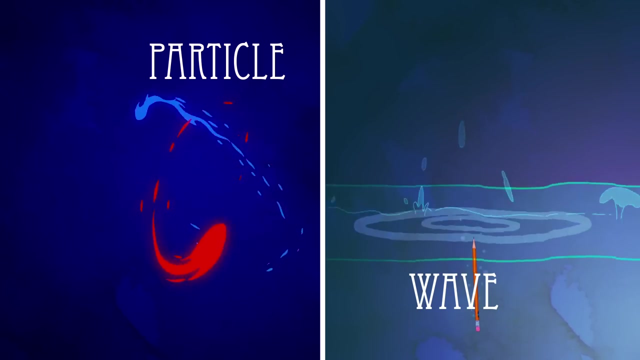 But what exactly is the stuff that's emitted from the sun and how do we see it? Is it a particle like atoms, Or is it a wave, like ripples on the surface of a pond? Scientists in the modern era would spend a couple of hundred years figuring out the answer to this. 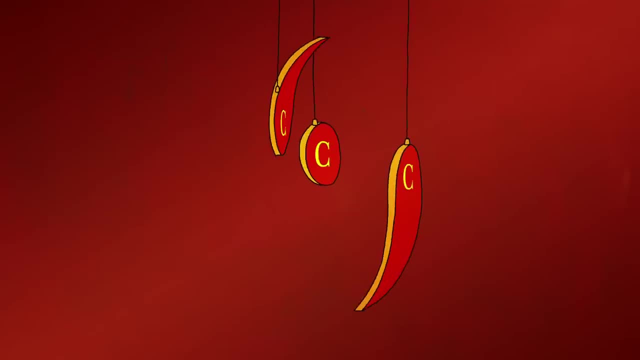 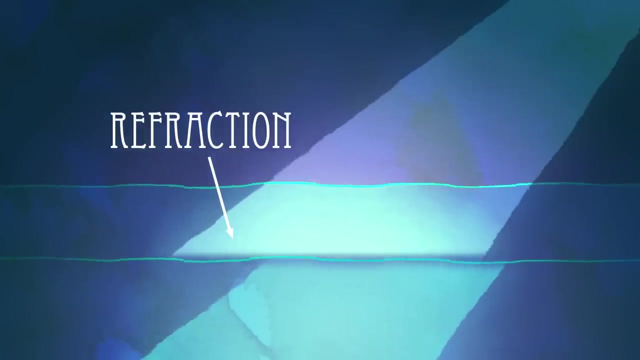 question. Isaac Newton was one of the earliest. Newton believed that light is made up of tiny atom-like particles, which he called corpuscles. Using this assumption, he was able to explain some properties of light, For example refraction, which is how a beam of light appears to bend as it passes from air into water. 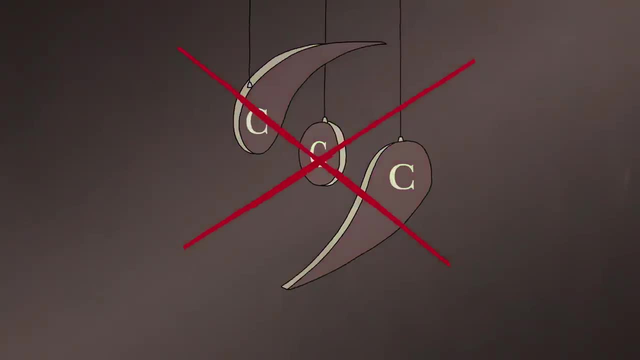 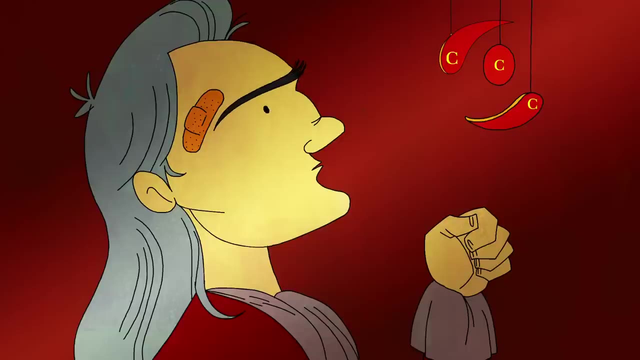 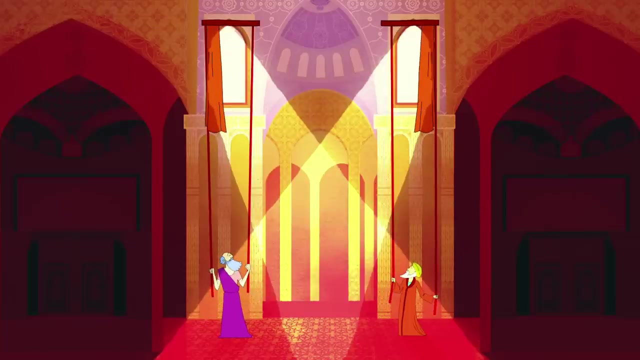 But in science even geniuses sometimes get things wrong. In the 19th century, long after Newton died, scientists did a series of experiments that clearly showed that light can't be made up of tiny atom-like particles. For one thing, two beams of light that cross paths don't interact. 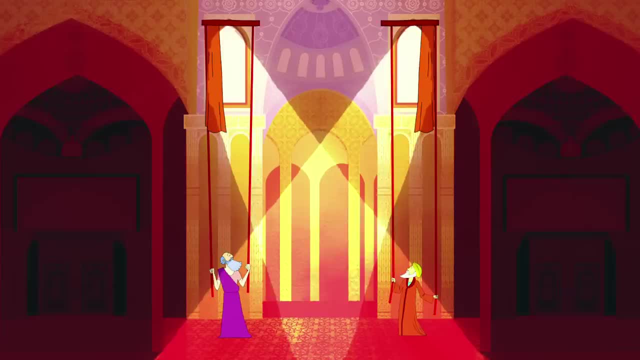 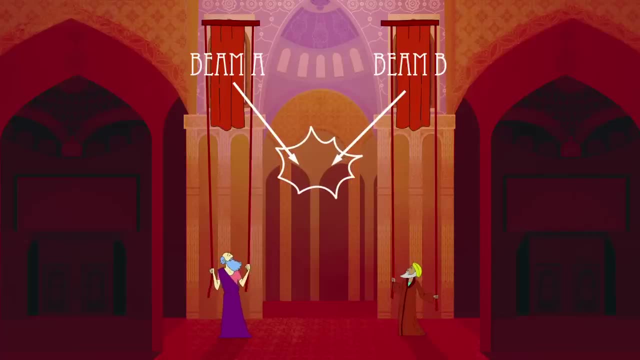 with each other at all. If light were made of tiny, solid balls, then you would expect that some of the particles from beam A would crash into some of the particles from beam B. If that happened, the two particles involved in the collision would bounce off in random directions. 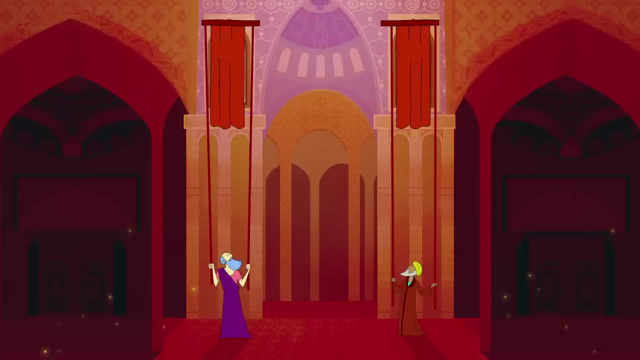 But that doesn't happen. The beams of light pass right through each other, as you can check for yourself with two laser pointers and some chalk dust. For another thing: light makes interference patterns. This means that light can be made up of tiny atom-like particles, For example, if you're 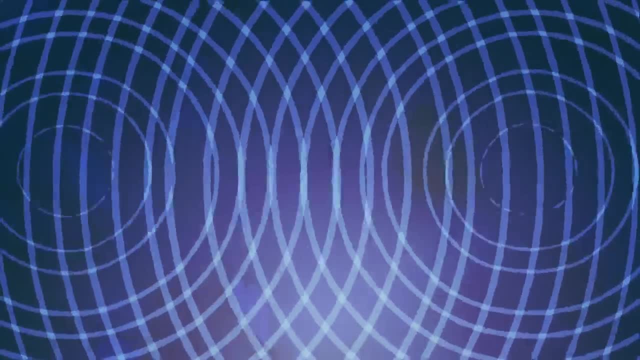 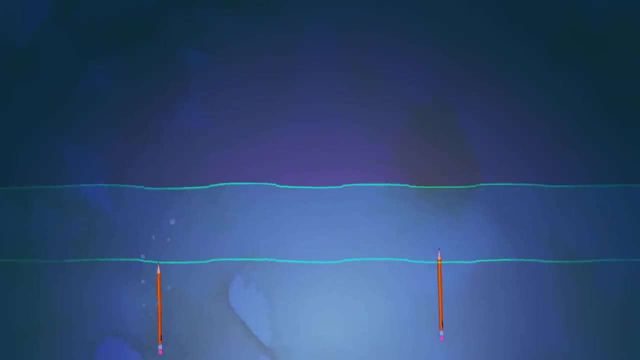 making interference patterns. light can be made up of two wave patterns. Interference patterns are the complicated undulations that happen when two wave patterns occupy the same space. They can be seen when two objects disturb the surface of a still pond and also when two point-like sources. 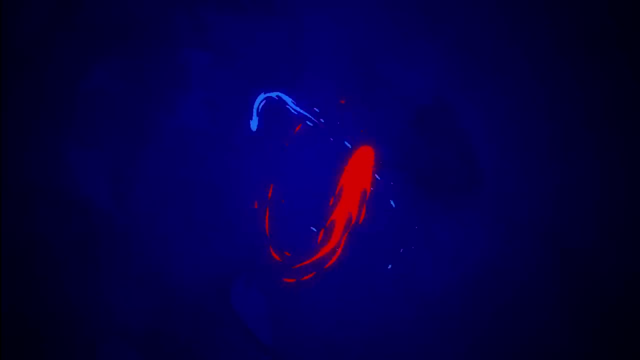 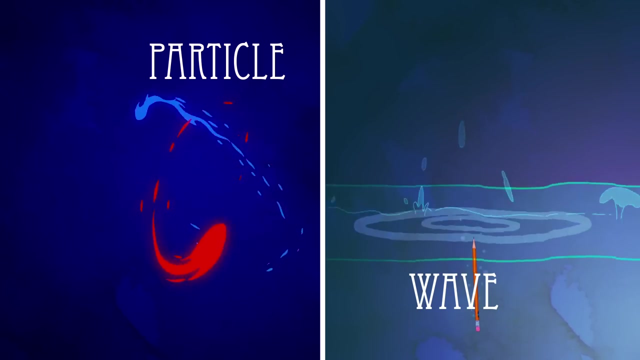 But what exactly is the stuff that's emitted from the sun and how do we see it? Is it a particle like atoms, Or is it a wave, like ripples on the surface of a pond? Scientists in the modern era would spend a couple of hundred years figuring out the answer to this. 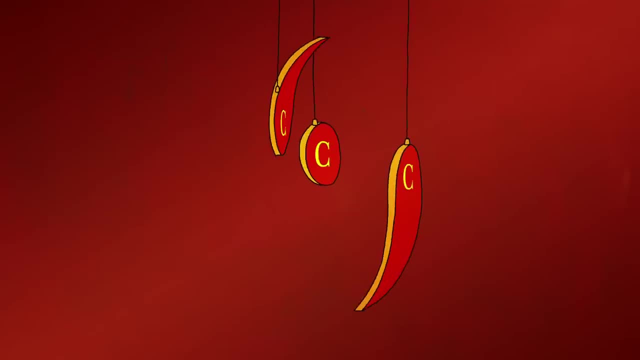 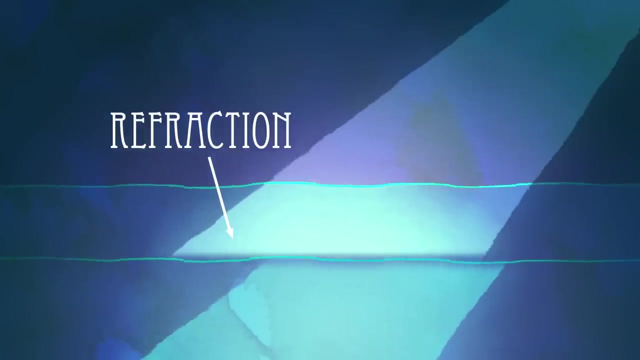 question. Isaac Newton was one of the earliest. Newton believed that light is made up of tiny atom-like particles, which he called corpuscles. Using this assumption, he was able to explain some properties of light, For example refraction, which is how a beam of light appears to bend as it passes from air into water. 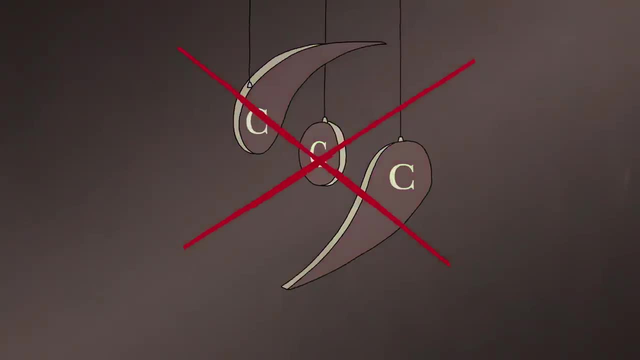 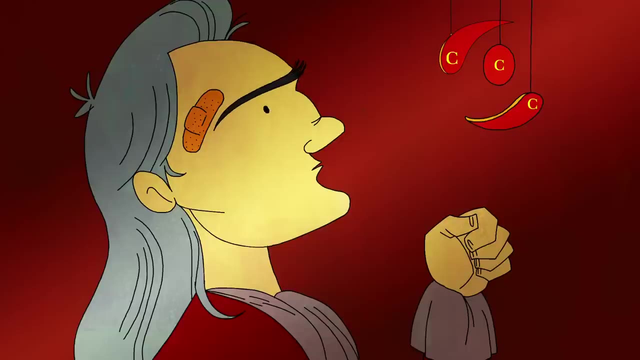 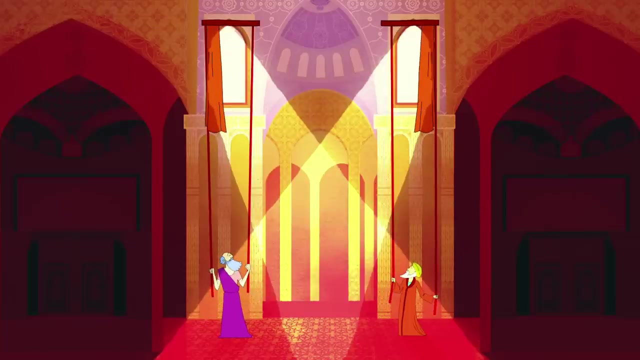 But in science even geniuses sometimes get things wrong. In the 19th century, long after Newton died, scientists did a series of experiments that clearly showed that light can't be made up of tiny atom-like particles. For one thing, two beams of light that cross paths don't interact. 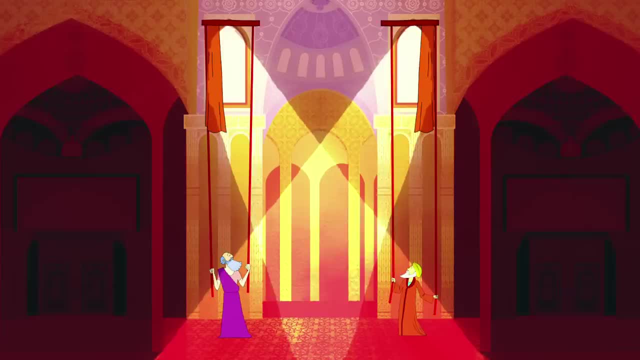 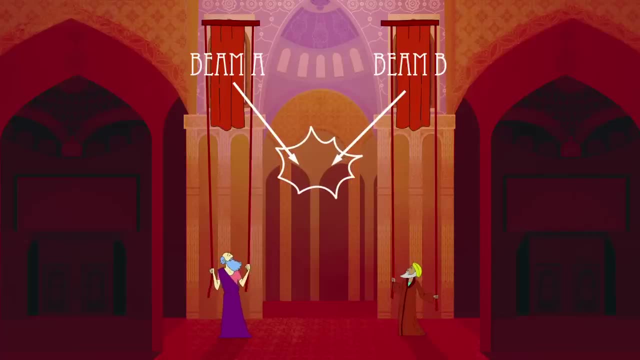 with each other at all. If light were made of tiny, solid balls, then you would expect that some of the particles from beam A would crash into some of the particles from beam B. If that happened, the two particles involved in the collision would bounce off in random directions. 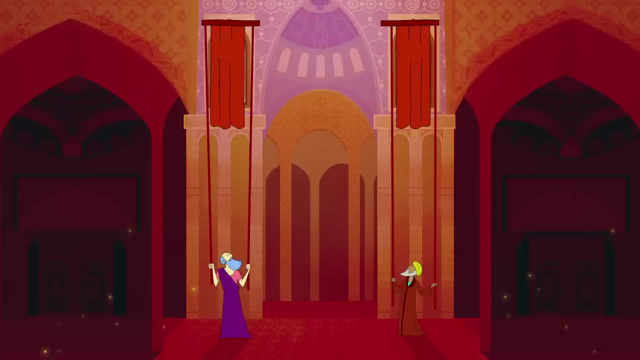 But that doesn't happen. The beams of light pass right through each other, as you can check for yourself with two laser pointers and some chalk dust. For another thing, light makes interference patterns. If light passes through a beam A, it will bounce off in random directions. If light passes, 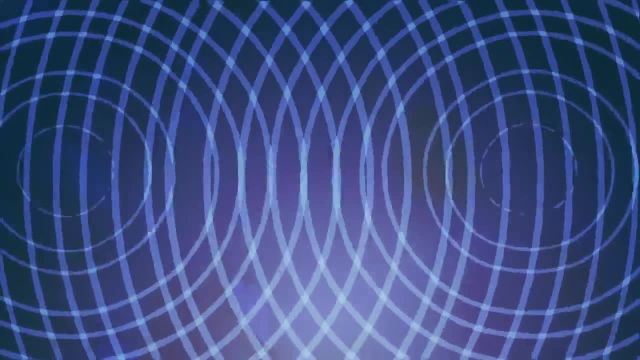 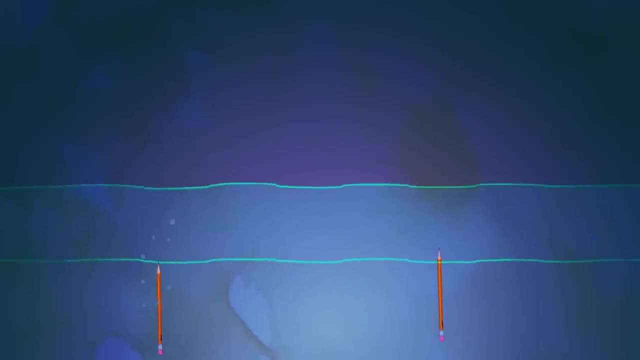 through a beam B, it will bounce off in random directions. Interference patterns are the complicated undulations that happen when two wave patterns occupy the same space. They can be seen when two objects disturb the surface of a still pond and also when two 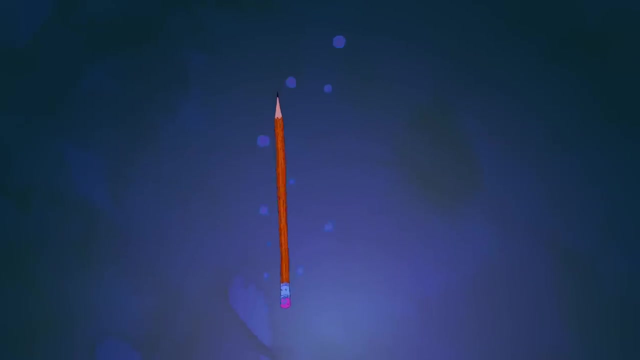 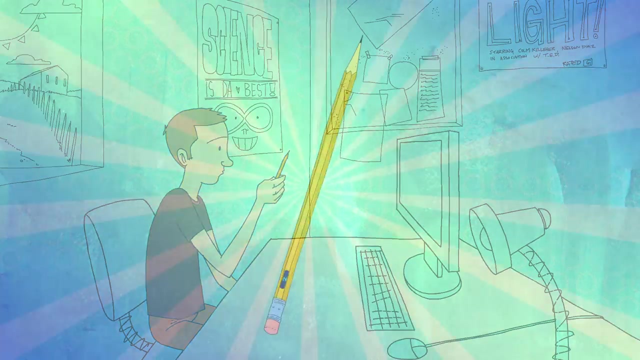 point-like sources of light are placed near each other, Only waves make interference patterns, particles don't. And as a bonus, understanding that light acts like a wave leads naturally to an explanation of what colour is and why that pencil looks yellow. So it's settled then. 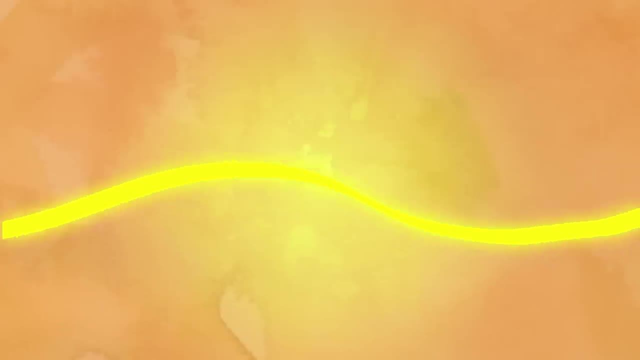 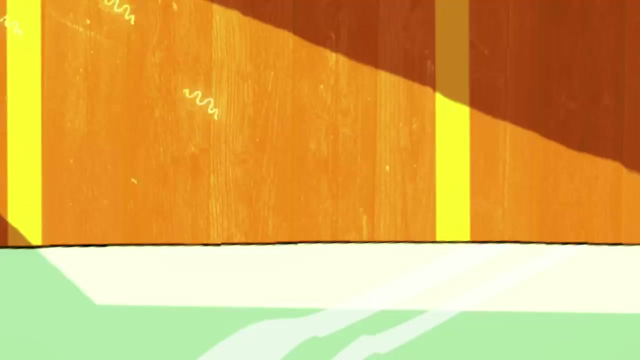 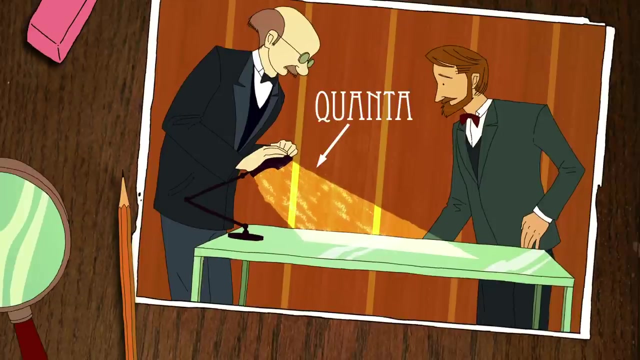 light is a wave right, Not so fast. In the 20th century, scientists did experiments that appeared to show light acting like a particle. For instance, when you shine light on a metal, the light transfers its energy to the atoms in the metal in discrete packets called quanta. But we can't just forget about properties.